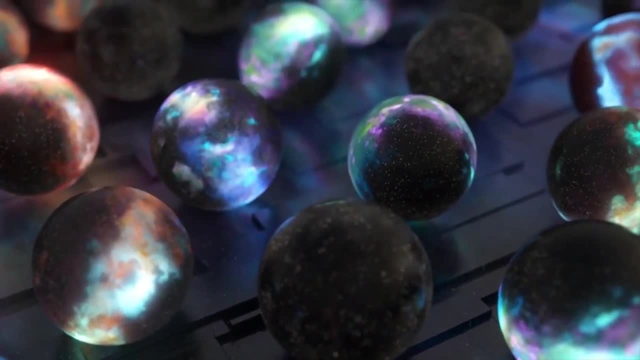 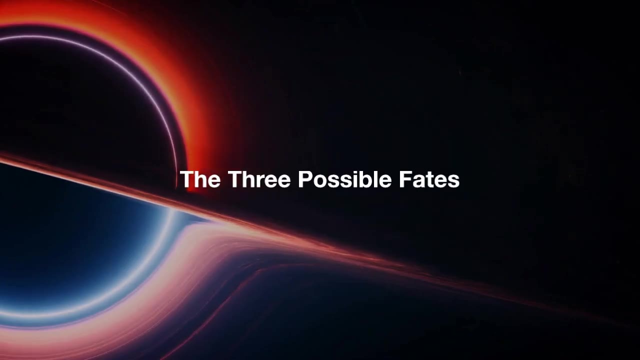 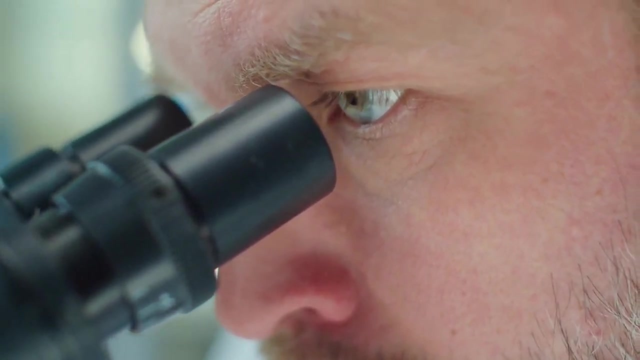 repulsive force pushing everything in the universe apart at an ever-increasing rate. These unseen forces hold the key to understanding the universe's ultimate fate: The Three Possible Fates. Based on our current understanding, there are three main possibilities for the ultimate fate of the. 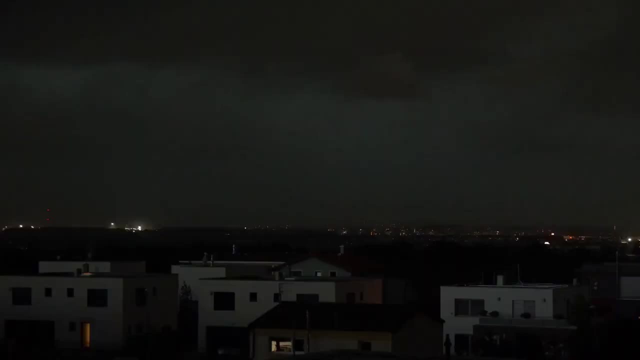 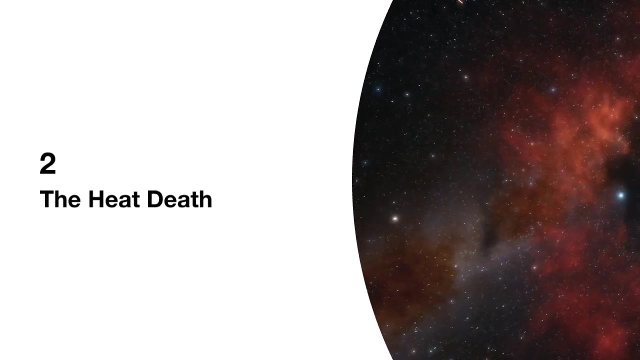 universe. 1. The Big Rip: If dark energy continues to strengthen its repulsive force could become so powerful that it rips apart the very fabric of space-time, tearing apart atoms and ultimately leading to the universe's complete disintegration. 2. The Heat Death. 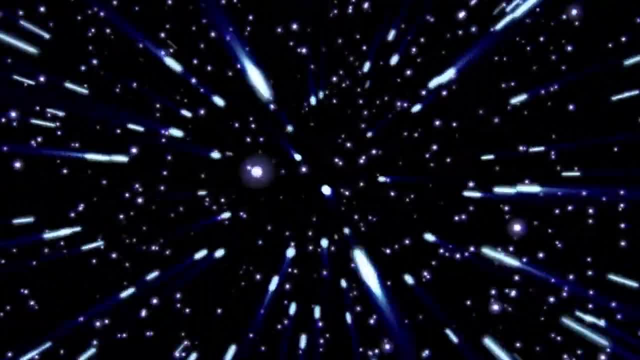 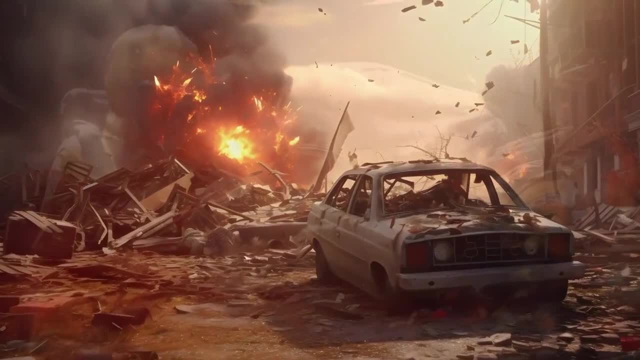 If dark energy remains constant or weakens slightly, the universe will likely continue to expand forever. Over time, stars will burn out, galaxies will disperse and the universe will become a cold, dark and empty place. 3. The Big Crunch. 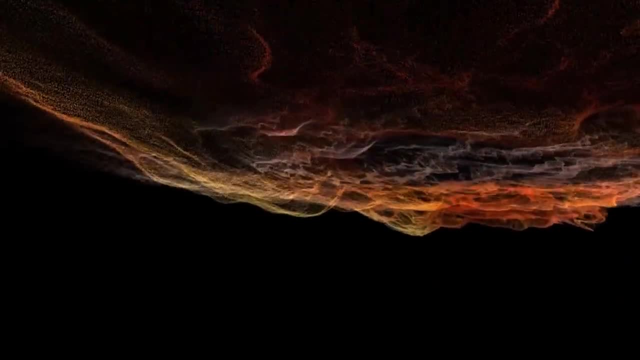 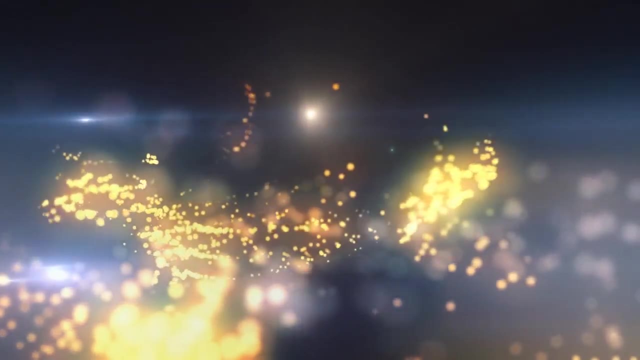 In this scenario, the density of the universe is high enough for gravity to eventually overcome the expansion, The universe will begin to contract, pulling galaxies back together in a fiery big crunch, potentially leading to a new big bang in a cyclical universe Unveiling the unknown. 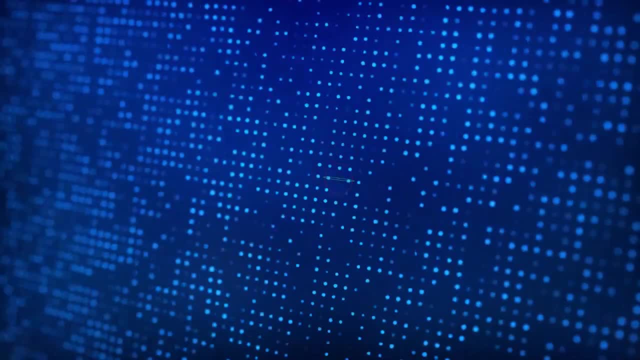 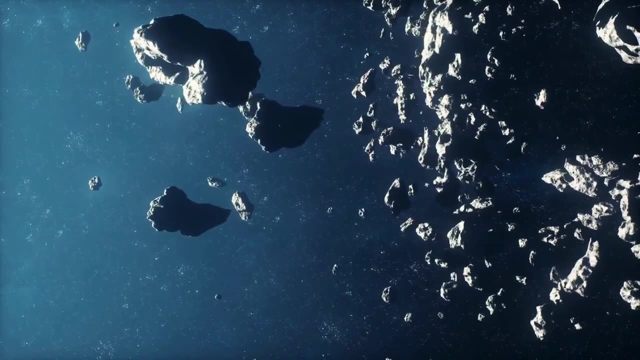 the role of dark energy. Unfortunately, we don't know enough about dark energy to say for certain which fate awaits us. Is it a constant force or is it changing over time? Understanding dark energy's nature is crucial to predicting the universe's ultimate destiny. 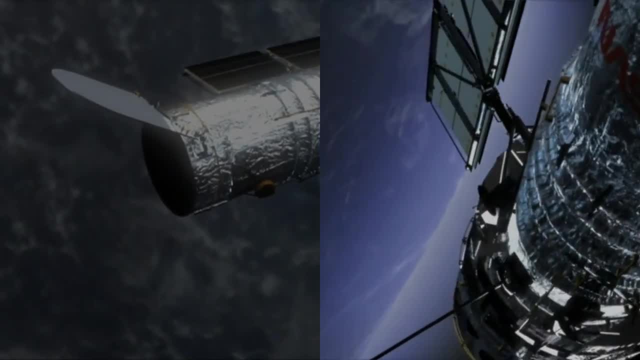 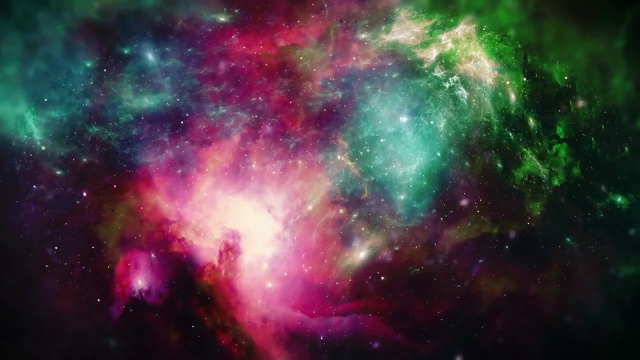 Powerful telescopes like Hubble and upcoming missions like the Euclid Space Telescope are designed to gather more data on dark energy and its influence on the expansion. Beyond our observations: the implication of other dimensions. Beyond our observations: the implication of other dimensions. 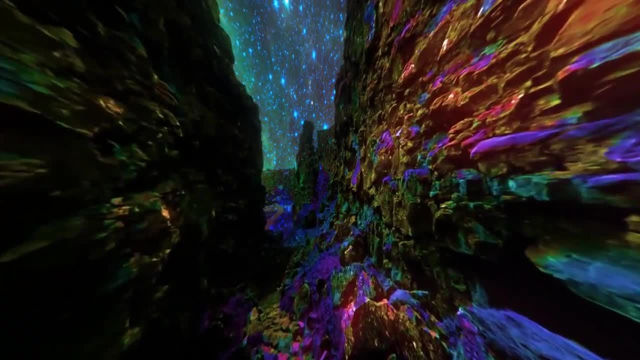 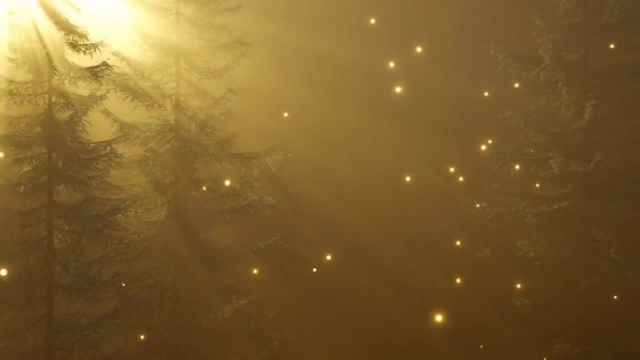 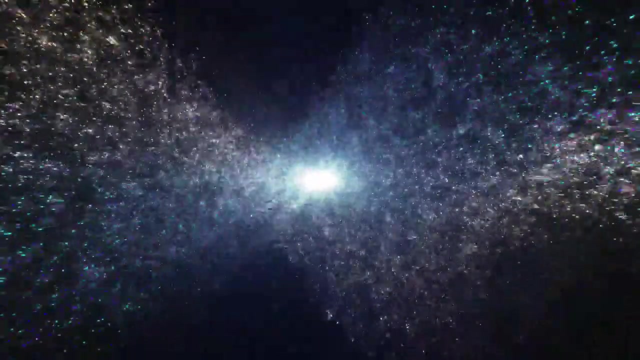 Some theories suggest the existence of additional dimensions beyond the three spatial dimensions and one-time dimension we experience. The properties and dynamics of these extra dimensions could also play a role in the fate of our universe. While these ideas are highly speculative, they highlight the limitations of our current understanding and the potential for mind-blowing discoveries in the future. 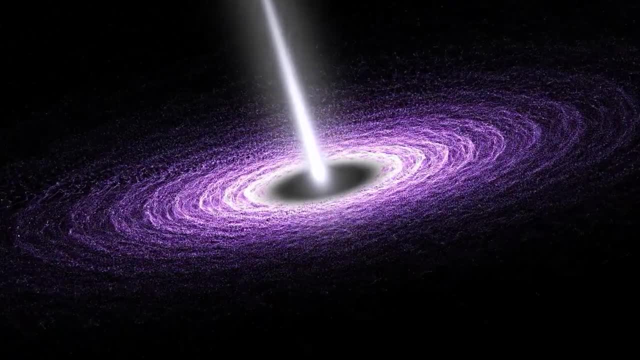 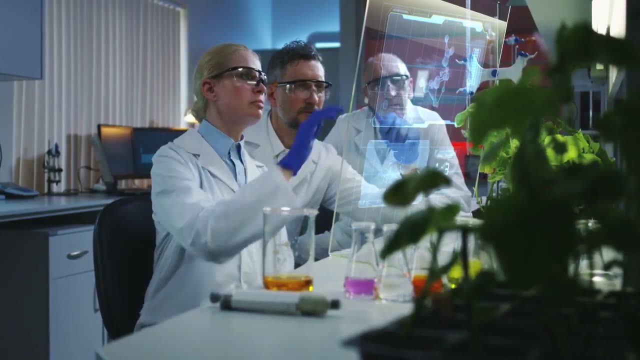 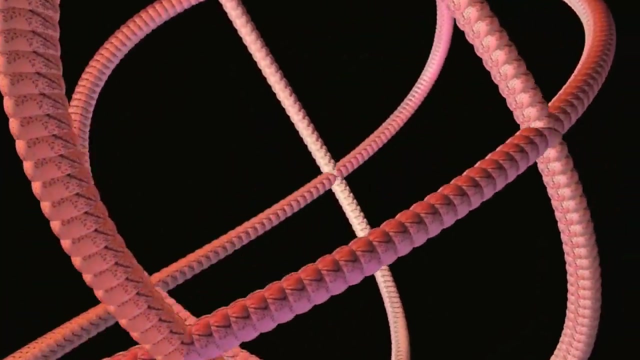 The Search for Answers Beyond the Standard Model. Unveiling the ultimate fate of the universe lies in pushing the boundaries of our knowledge. Physicists are constantly searching for a theory beyond the standard model that can explain dark matter, dark energy and the nature of gravity on a grand scale.